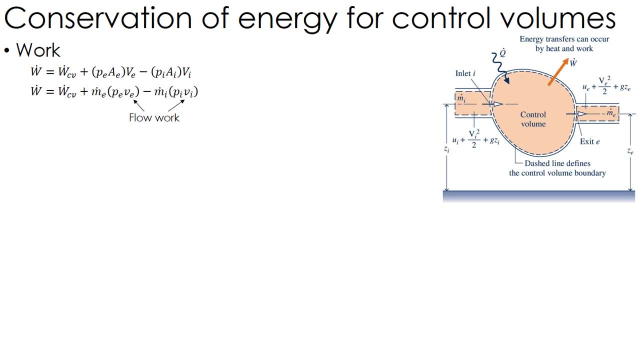 again times our mass flow. So that's a flow work which is separate from the work that's being done by spinning a blade or something like that. Including this flow work into our first law energy balance equation, this is basically again a time derivative of our first law equation. So 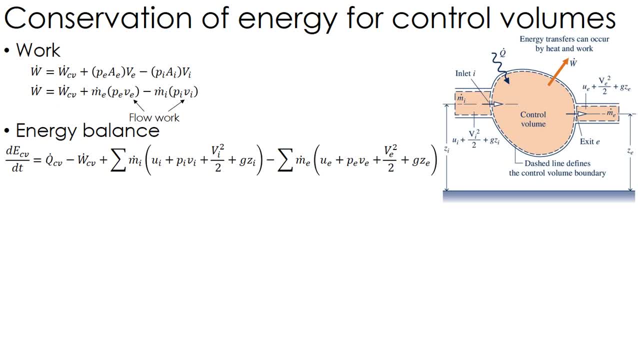 the change in energy with respect to time again is rate of heat transfer minus the rate of the work. Again, this is the work of the control volume. Then I have my u values, my kinetic energy, my potential energy, and I also have this flow work pv that I've included in there as well. 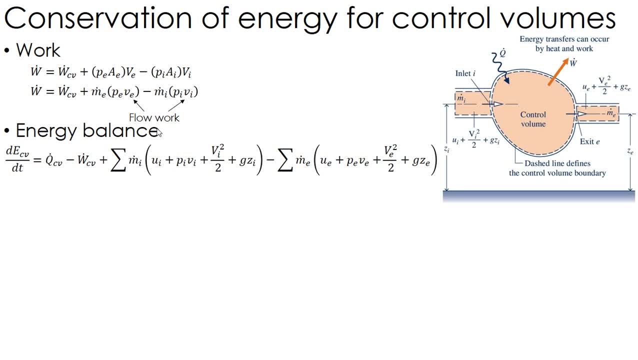 So I've got this extra term, this pv term, and that's just from the fact that there's some work due to the fact that I've got flow going on here right Now. if you remember, we talked about enthalpy right, And we just kind of said, hey, by definition, enthalpy is u. 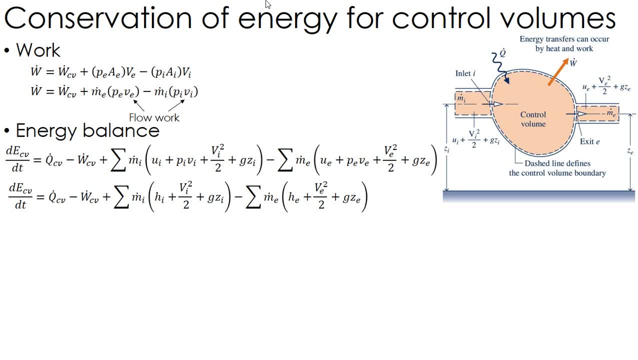 plus pv. We'll talk about why it's important later. This is why it's important because I don't want to have to look up u, pressure and volume and then do a calculation. I just want to look up h directly, So that's really where enthalpy comes from. It just makes our calculation. 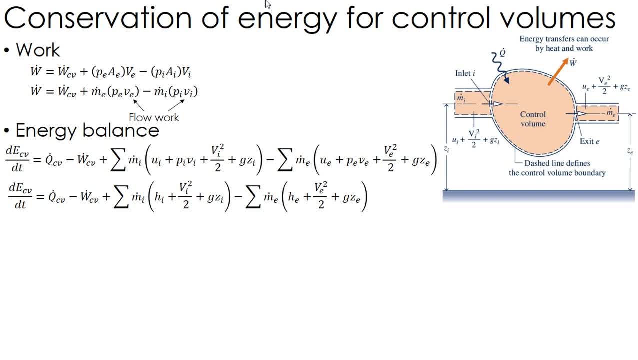 easier. okay, It doesn't have a huge physical meaning that you're going to be able to point at and say, oh, look at that enthalpy going on there. Again, it's a combination of variables that makes our life easier to do our energy balance to. 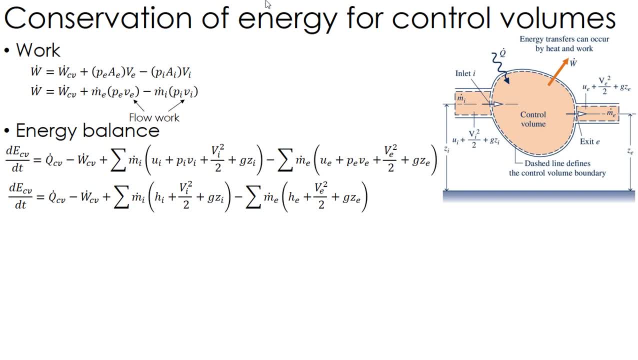 make the first law work out, okay. So, rather than spending a lot of your energy trying to figure out exactly what the physical definition of enthalpy is, just know that if I've got fluid flow, I look up h rather than looking up u, And h is nothing more than a collection of u plus pv. 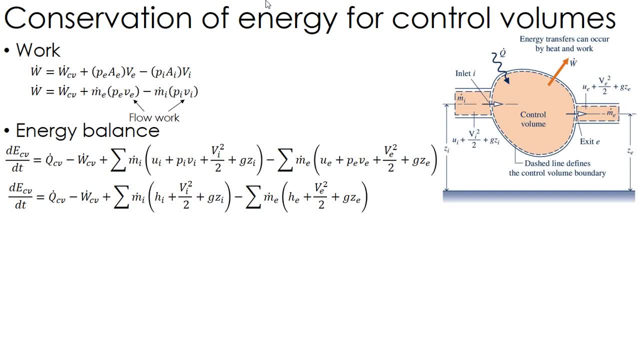 So, rather than calculating it, it's just tabulated to make our life easier, And we give it the arbitrary name enthalpy, which has physical meaning. that is not important. What's important is that this flow is not important. It's not important, It's not important, It's not important. 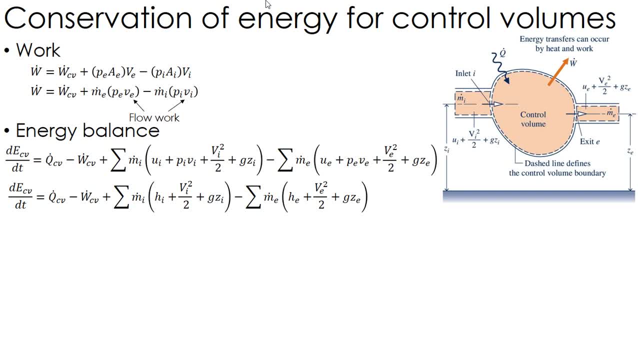 So our first law- energy balance- is used and that we use enthalpy because we've got this flow work for flowing control volume okay. Now in our problems we're dealing with steady state. Once this thing wraps up and ramps up to steady state, properties are not changing. Therefore, 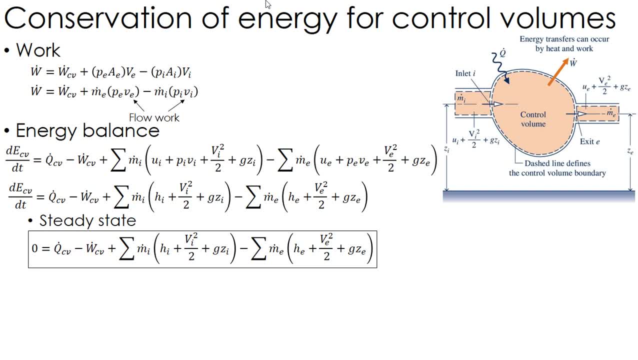 the change in energy does not change as a function of time. So the left side of the equation goes to zero And basically what I have is heat minus work plus enthalpy, And I'm going to go back to energy balance. So I'm going to go back to the first law- energy balance, and that we use enthalpy. 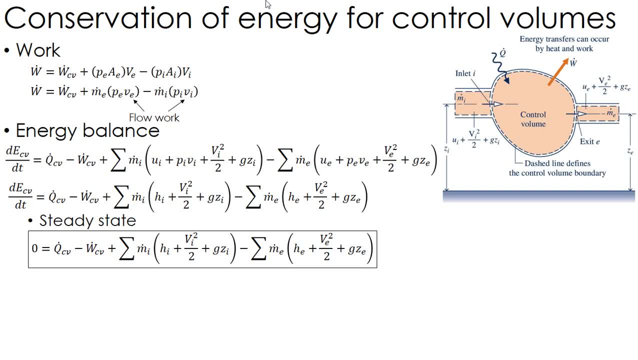 Energy in minus energy out, And that energy includes, you know, energy, flow, work, kinetic energy, potential energy, Although a lot of these are oftentimes neglected. Main thing to remember is, with a control vine, when I have flow, I need to look up H values, not U values when looking in tables. 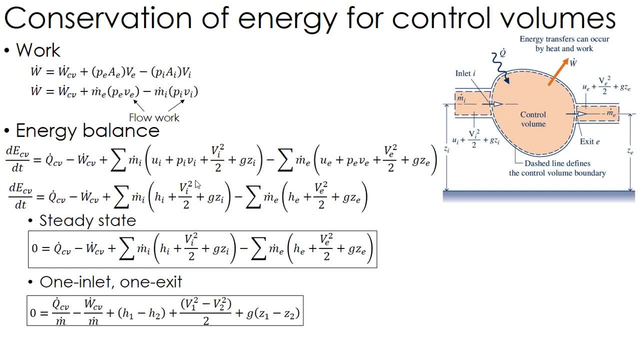 Okay Now, for a lot of our systems we have one inlet, one outlet. I can rewrite that. So, rather than the sum of everything coming in minus the sum of everything going out, it's basically, you know, inlet minus outlet. 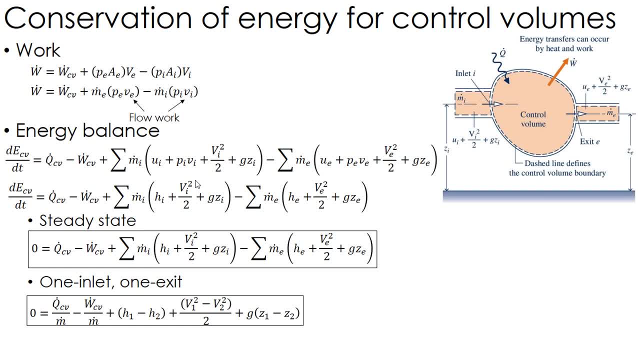 You know, one minus two is basically what I have here. Okay, And for a lot of our devices that's what we have, Probably 85% of the devices we use: one thing coming in, one thing going out. Now talk about these devices. 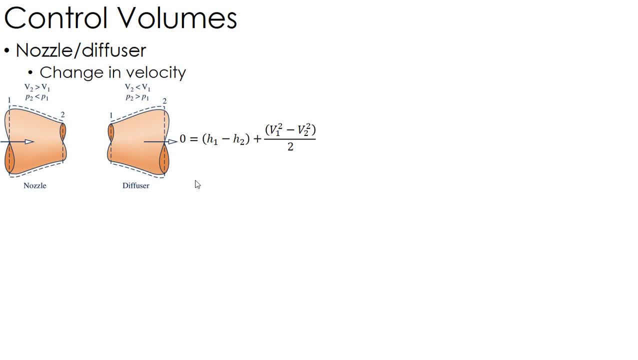 I'm going to step through them, talk a little bit about each one. So the first one I'm going to talk about is a nozzle or a diffuser. So a nozzle basically increases the velocity, A diffuser decreases the velocity. Okay, 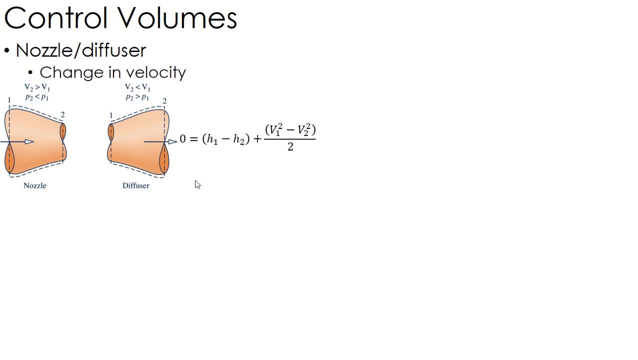 So really, there's no work here. There's no heat loss to the surroundings or heat gain from the surrounding. All that's really happening is I'm changing my kinetic energy. Okay, So basically, knowing the properties on both sides, I can calculate the enthalpy. 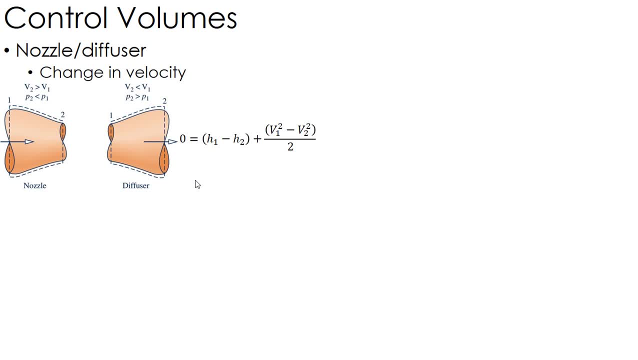 And then from that that change in enthalpy is essentially equal to the change in kinetic energy, which is again V squared over two. Okay, So that's. That's how you deal with a nozzle or a diffuser. Generally no work or heat transfer is just: delta H equals delta K E. 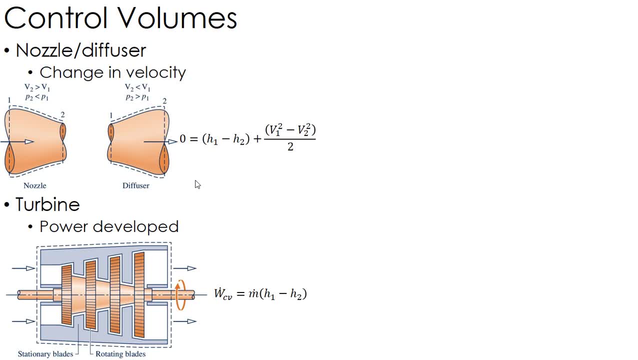 Okay, Most of the other things. K? E is ignored, just like P E is ignored, Okay. So next thing I want to talk about is a turbine. Okay, And the point of a turbine is you put in high energy fluid and get that energy out into the form of, you know, spinning a blade. 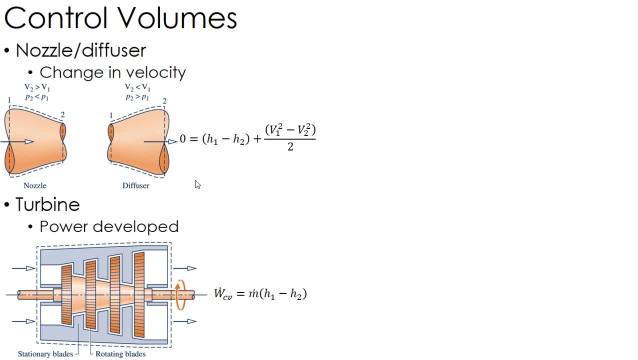 Okay, Um, generally, unless it states otherwise, turbines are adiabatic, So there's no heat loss. that goes away. Again, kinetic and potential energies are minuscule with compared to my change in enthalpy, So really just the work of a turbine, assuming it's adiabatic turbine, which is most turbines we're going to deal with. 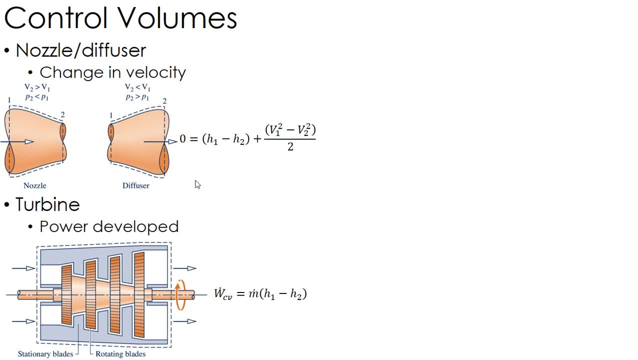 Really just the work of the turbine is just the change in enthalpy. So again, looking up the enthalpy, I can get the work just by the difference between the enthalpy. The opposite of a turbine is either Compressor, a pump, where I'm putting work into the system. 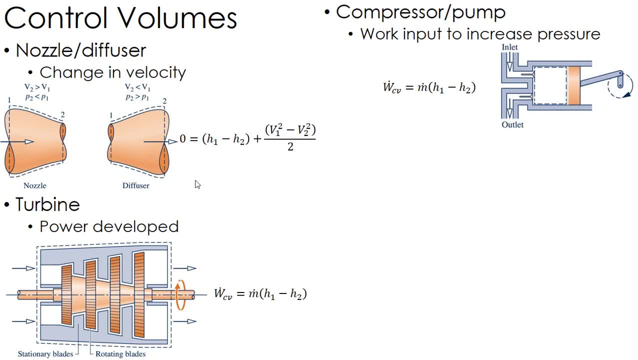 Okay, In order to get an increase in pressure, Okay. So again, we typically assume these are adiabatic, kinetic and potential energy are much smaller as compared to the change in enthalpy. So really, that work that you're putting in is just the change in enthalpy. 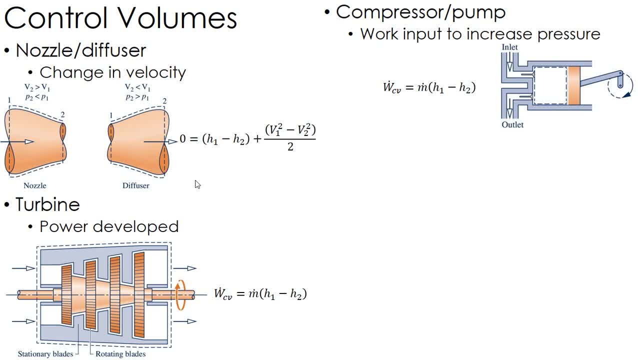 So, again, finding that enthalpy gives us the work, either the work out of a turbine or the work Into a compressor or pump. Okay, Now the other main thing that we have is a heat exchanger. Okay, And what a heat exchanger is? basically, you've got two or more streams of fluid. 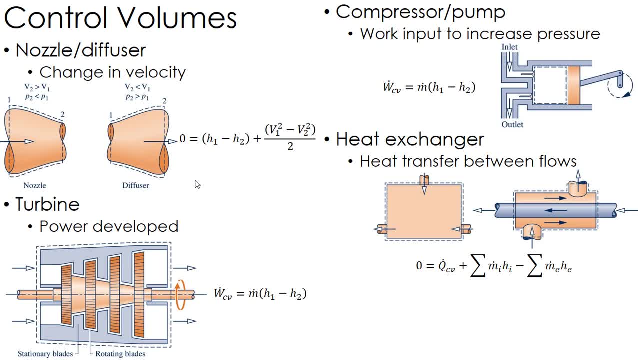 They have some sort of interaction where the heat between them is exchanged. Okay, So basically what you have is you have any heat loss to the surroundings, which oftentimes is zero, If you've got you know just, You know just the streams interacting, but then basically the enthalpy in minus the enthalpy out. 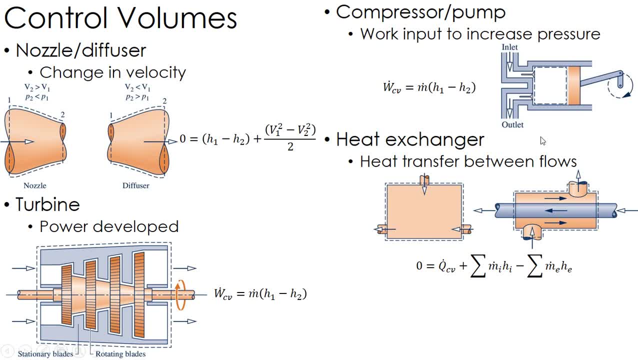 And again, if the container, if the control volume is insulated and it's just the interaction between the streams Right, So for example this one here on the left, I've got two streams coming in, They mix, and one goes out. 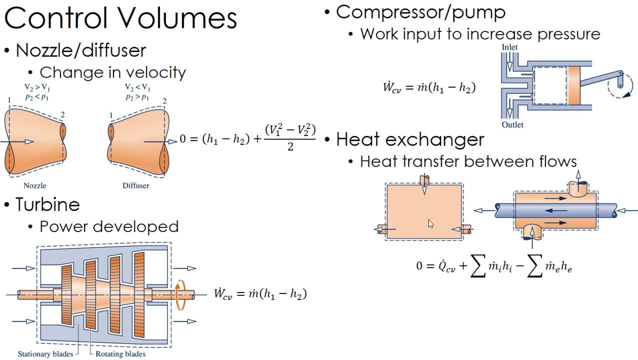 Q is zero to the surroundings. The only interaction is: the enthalpy in basically equals the enthalpy out. Okay, So a lot of it is just how you're Defining your system as to whether or not there's a Q to the surroundings or not.